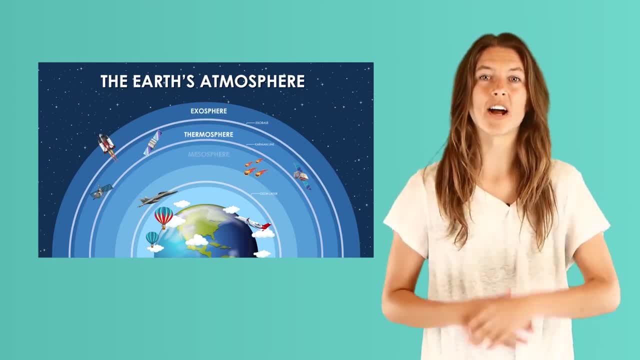 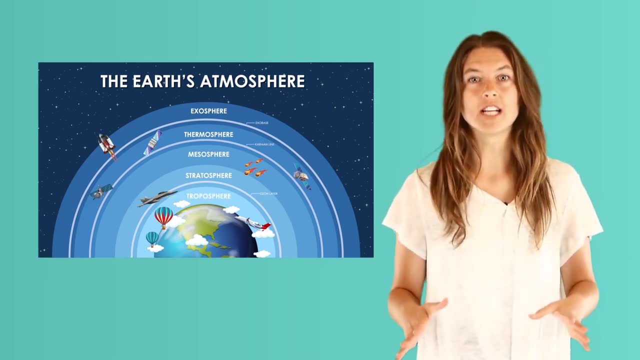 The atmosphere is layers of gases that surround the Earth. Weather happens in this layer and it's a gas. The atmosphere is layers of gases that surround the Earth's atmosphere, called the troposphere. Evaporation happens all the time without realizing it. 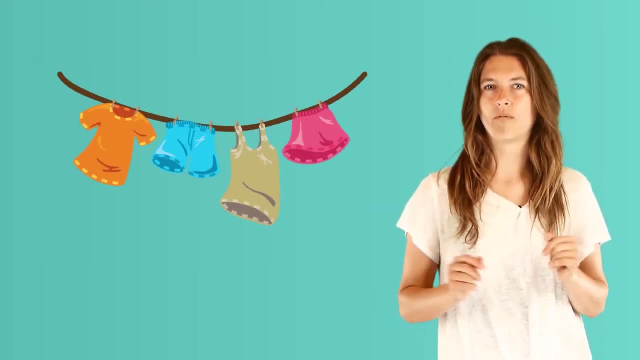 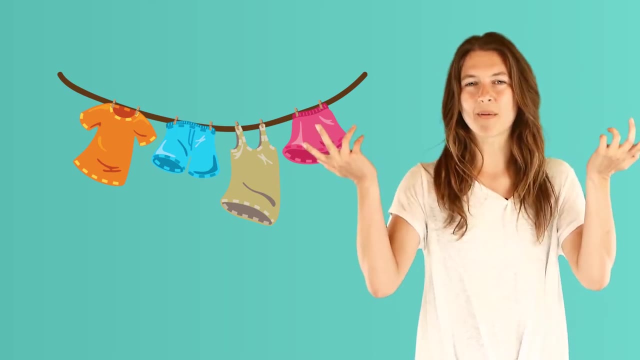 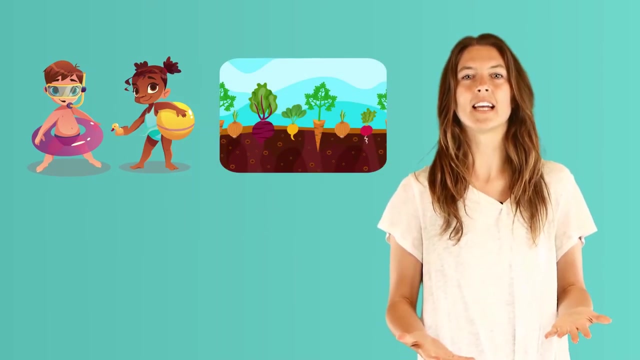 Do you ever hang your wet swimsuit out to dry in the sun? When your swimsuit goes from wet to dry, it's because the sun heats the water in the suit and it evaporates into vapor. The same is true for your wet hair after swimming or wet soil in your garden when the sun heats it after a rainfall. 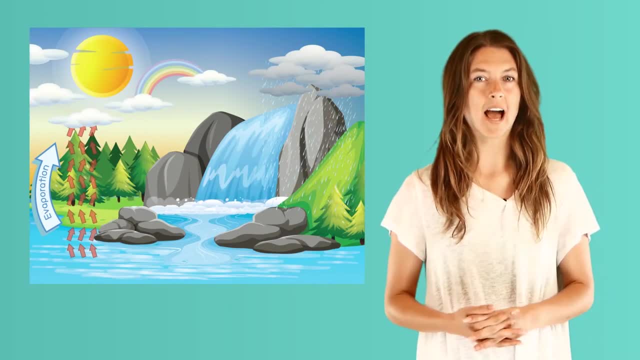 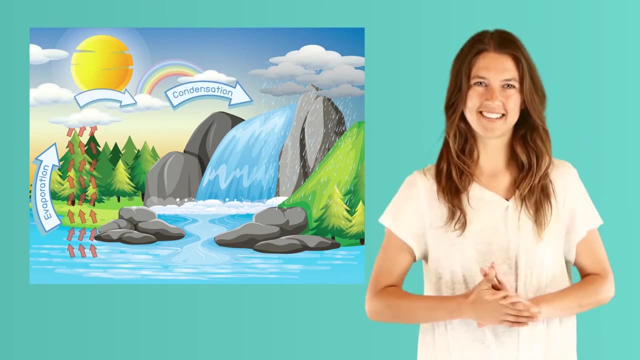 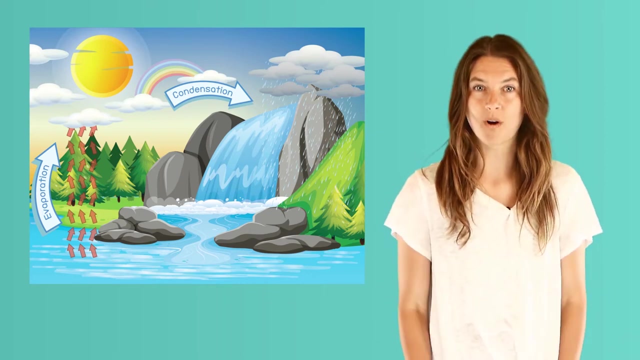 Do you know what water vapor becomes? Yes, When water vapor cools and condenses, it becomes a cloud. Condensation happens when the water vapor becomes liquid again and forms clouds. When too much water has condensed or turned into liquid droplets, the clouds become very heavy. 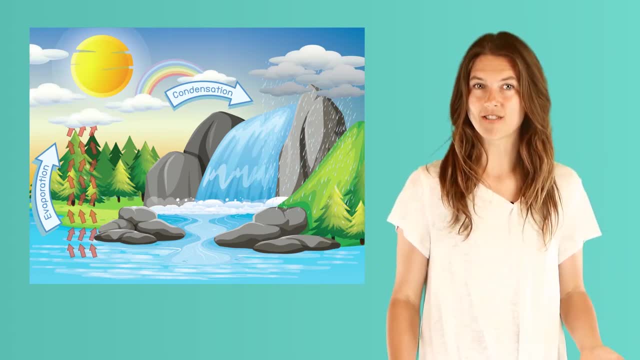 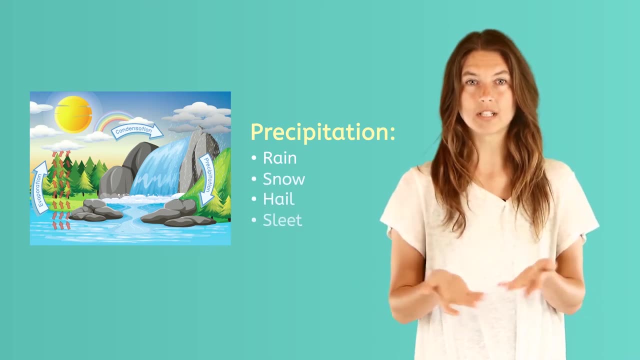 That's when water falls back down to the ground, called precipitation. Precipitation is a big word that really means rain, snow or rain. Precipitation is a big word that really means rain, snow or rain. It's not snow, hail or sleet. 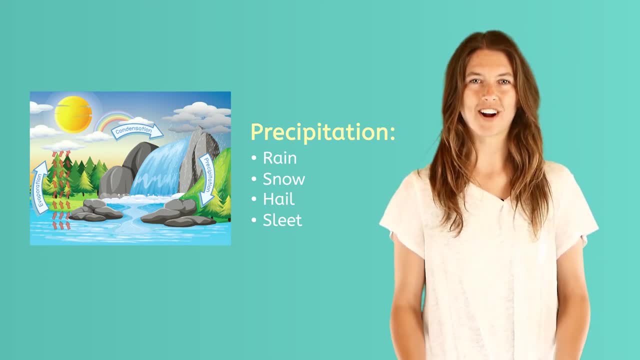 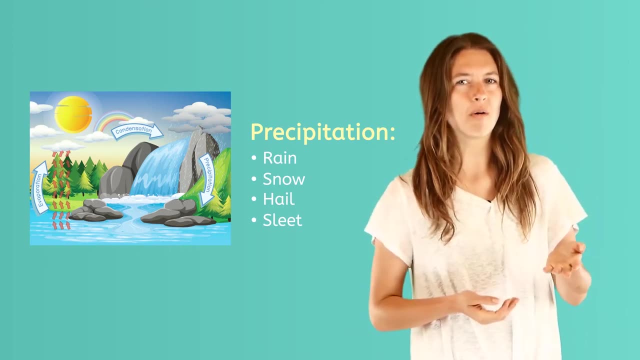 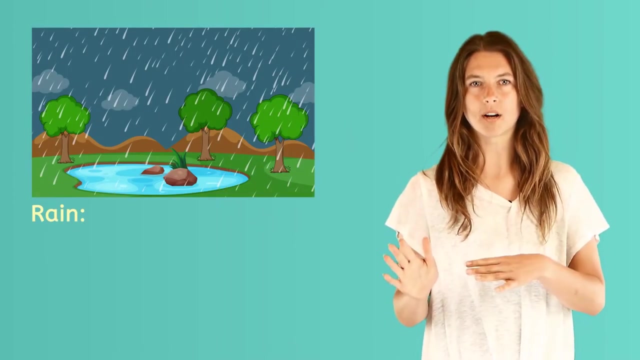 It's the liquid and water particles that fall from the clouds onto the ground. But why does precipitation sometimes come down as rain, other times as snow or hail or sleet? Let's look at this process more closely. Rain is a water vapor from the air that condenses and falls as water droplets. 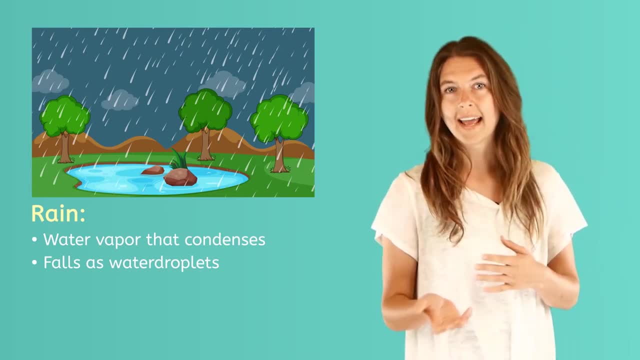 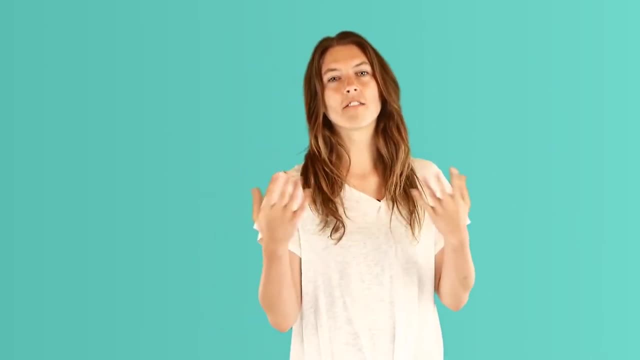 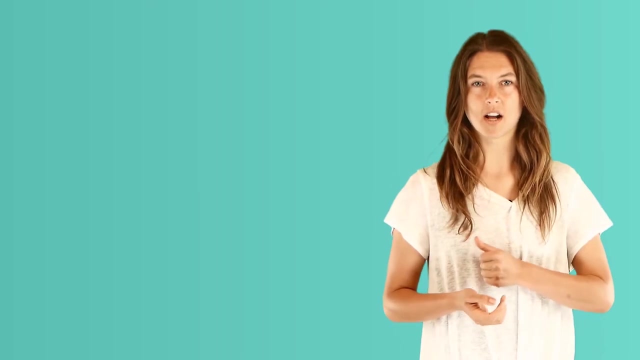 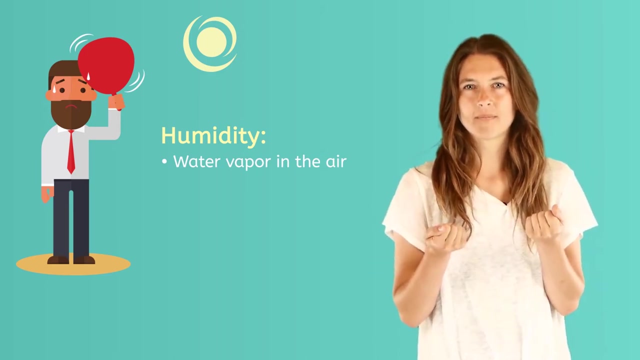 It provides water for plants and animals. It helps a garden grow, helps fill ponds and streams. When light reflects on water droplets in the air, it creates a colorful spectrum called a rainbow. In hot weather, you might hear adults talk about humidity. Humidity is water vapor in the air and it makes your skin feel moist, Do you? 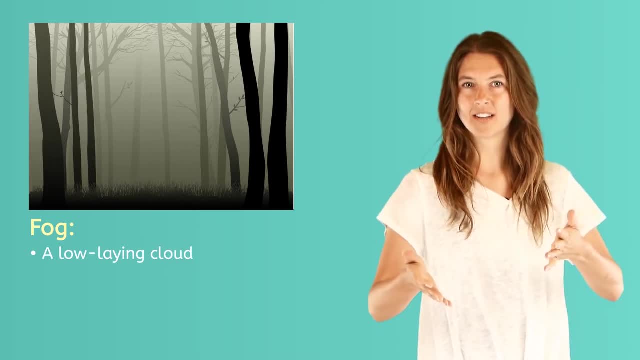 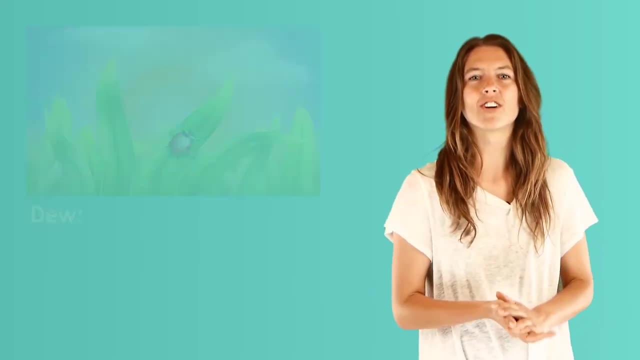 know that fog is cloud in the air near the ground. Yes, When you wake up on a foggy day, you're actually in a cloud. On summer mornings, you might wake up and find that the grass is wet without having rained or without the sprinklers being on. That's because during 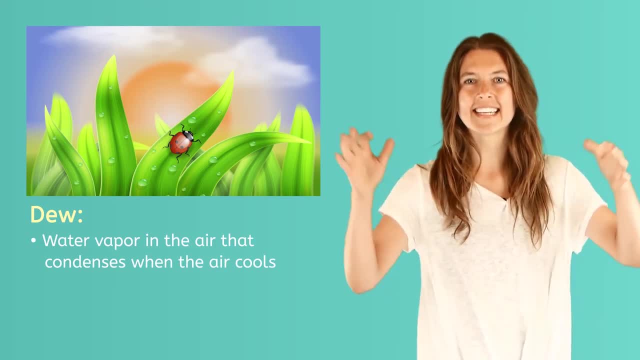 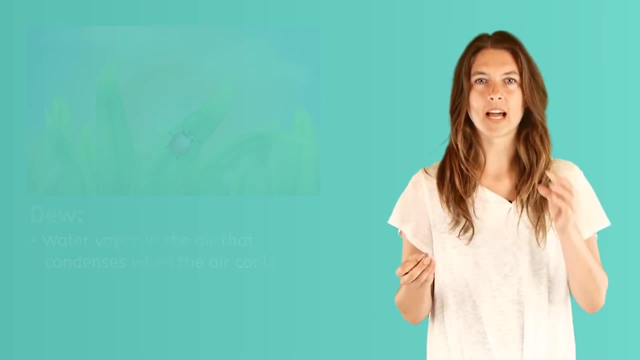 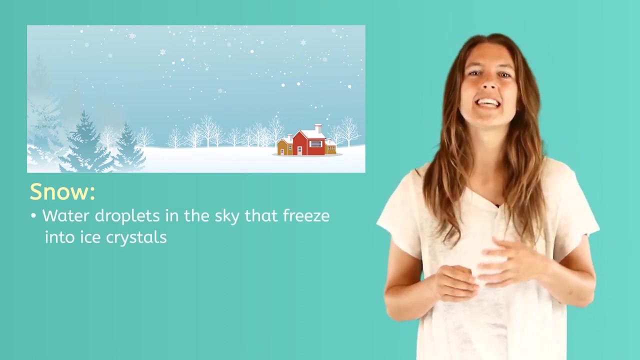 the night, the air is cool and the water vapor in the air condenses onto the ground and the plants. This moist surface it creates is called dew. Now, snow is water droplets in the sky that freeze into ice crystals before they fall to the ground. This happens when temperatures 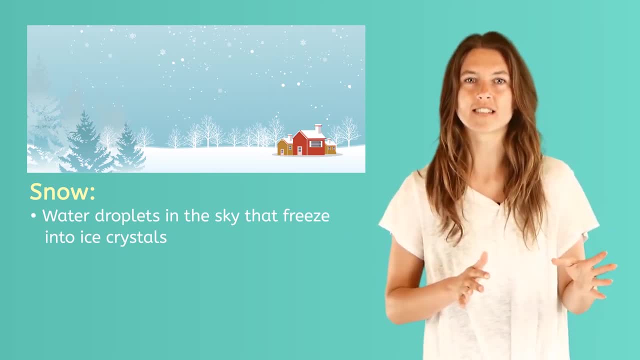 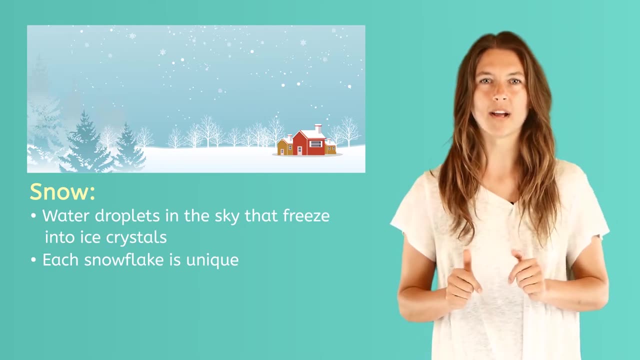 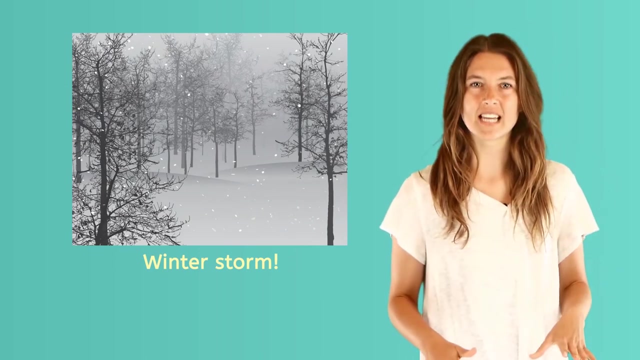 are so cold that you can't even breathe. This is called dew. Snowflakes are unique. Even though every snowflake has six points, no two snowflakes are alike. A major winter storm consists of a lot of snow, freezing temperatures and. 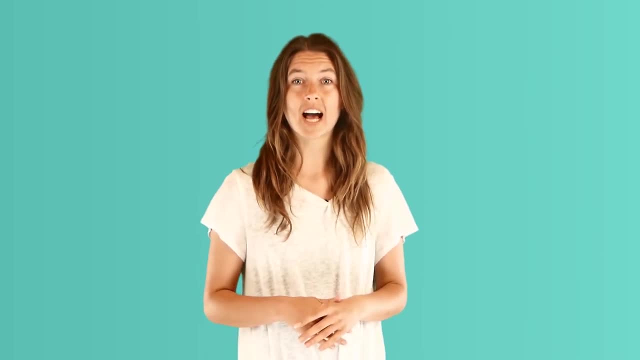 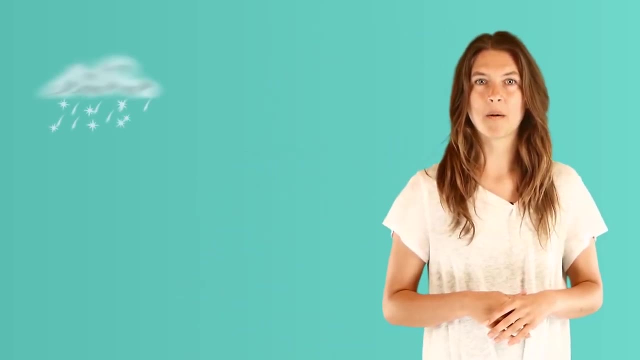 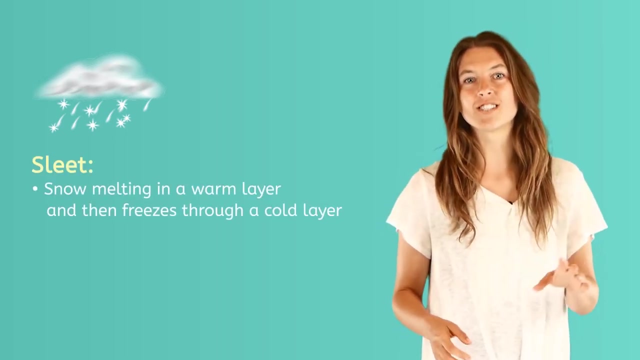 high-speed winds. Sometimes water droplets in the clouds don't come down as raindrops or snowflakes. Sometimes they are ice pellets. When the snow melts in a warm light, the snow melts in a warm layer and then refreezes into ice as it comes through a cold layer. 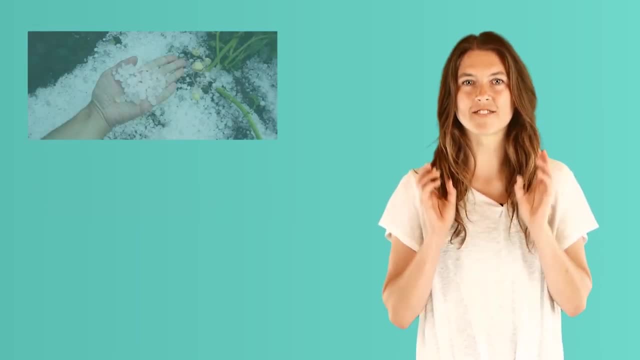 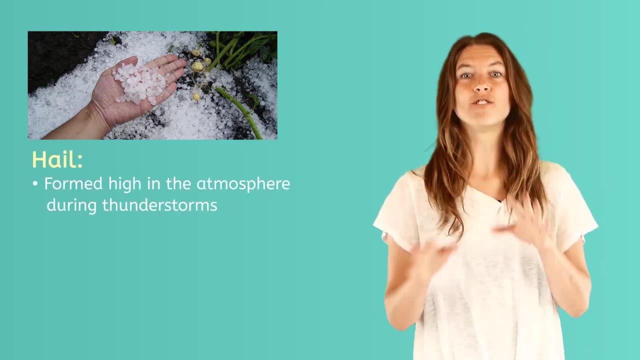 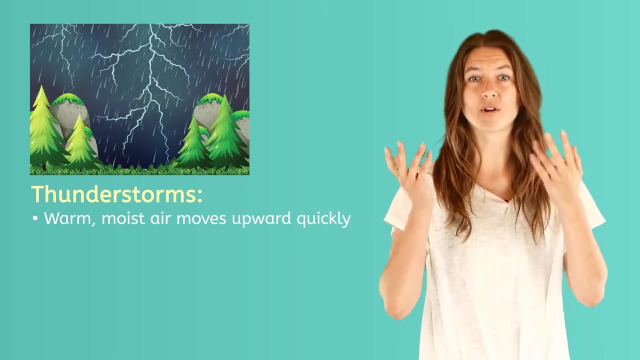 It is known as sleet. When the water droplets freeze in warmer temperatures, like in spring or summer, they come down as hail. Hail is usually formed in the clouds during thunderstorms. Thunderstorms happen when warm, moist air moves upward really fast. When this fast-moving air cools and condenses. this then becomes snow. This then becomes clouds. The water droplets can sometimes become ice. As the ice pellets come down, they bump into other ice pellets and other water droplets. They become larger ice pellets until the cloud can no longer hold them at all and they fall like hail. 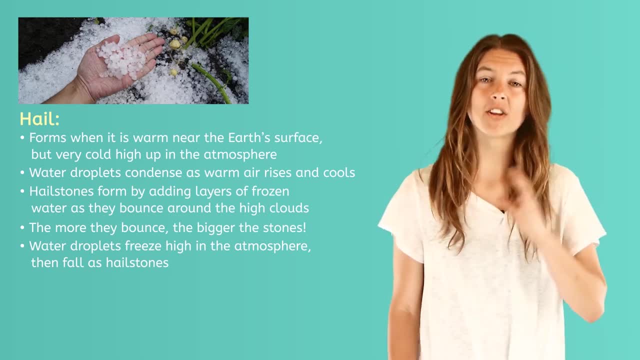 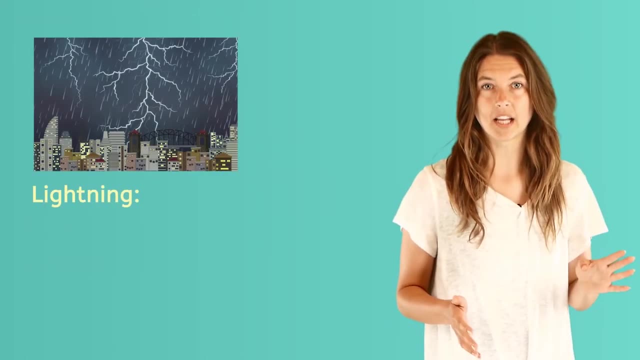 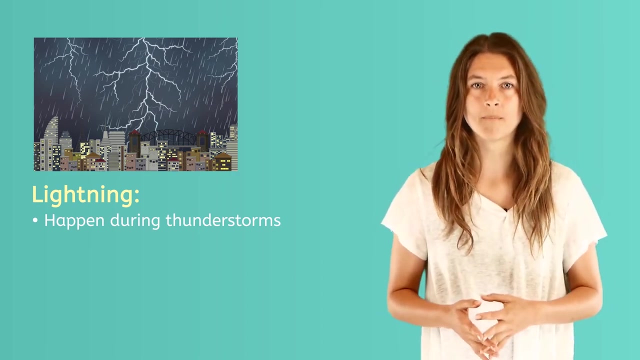 on the earth's surface. The more they bump around, the bigger the hail, storm, Thunderstorms and lightning go hand in hand. When the air is hot, it can drop ice, and lightning happens during every thunderstorm. you cannot have thunder without lightning. lightning is electricity produced by all those ice. 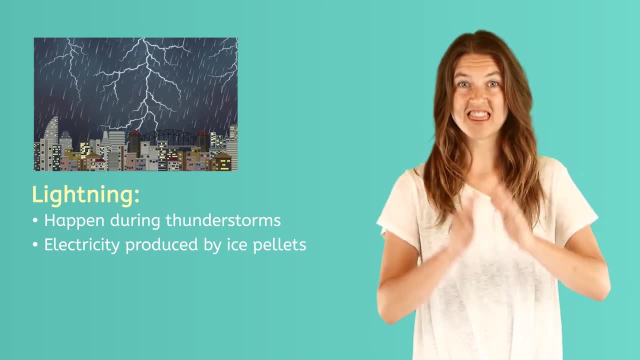 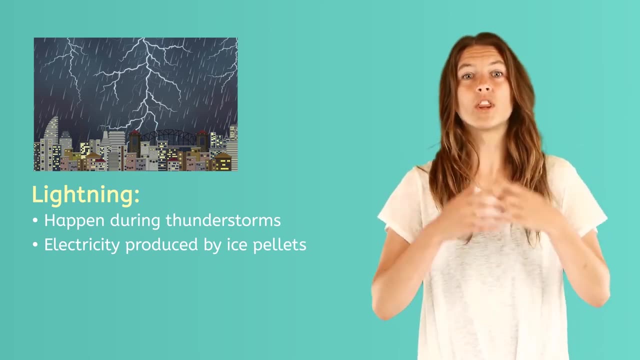 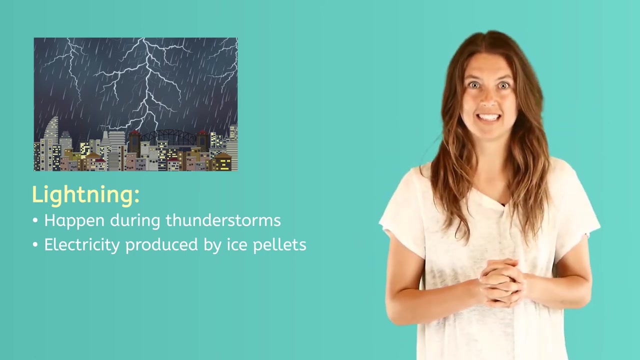 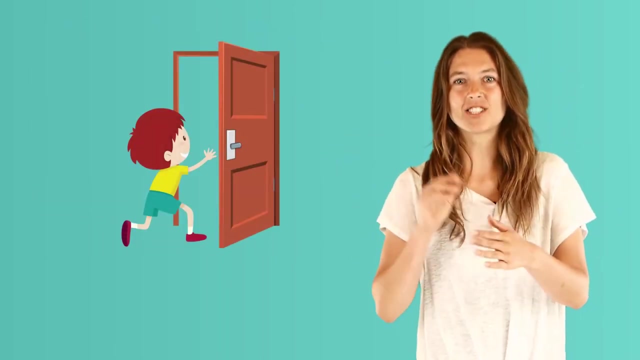 pellets in the sky that bump into each other, they create electrical charges that eventually fill up the entire cloud. then that cloud charge connects with a huge charge on the earth, like trees or the ground, and then zap, lightning strikes- ouch. have you ever rubbed your feet on a rug and then touched a metal? 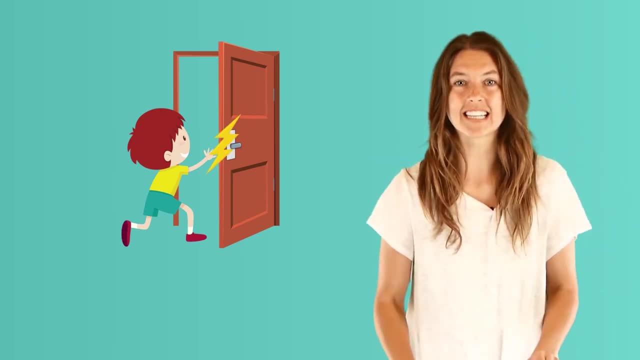 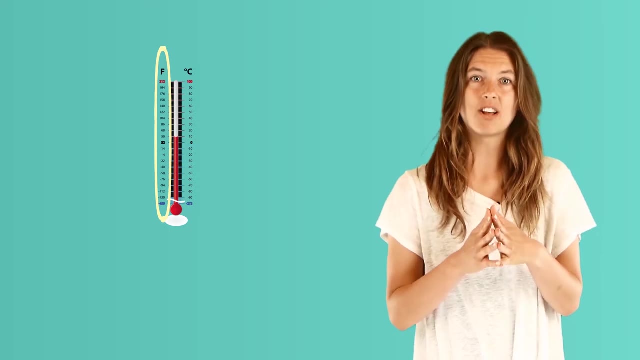 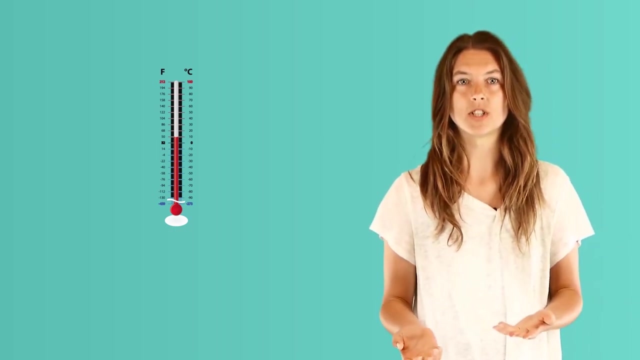 doorknob or something and it zaps you yikes. it's just like lightning. lightning can be as hot as 54,000 degrees Fahrenheit. Fahrenheit is a scale used to measure temperature. that's how we in the USA record daily weather temperatures, but most countries use the centigrade scale and record temperature in.